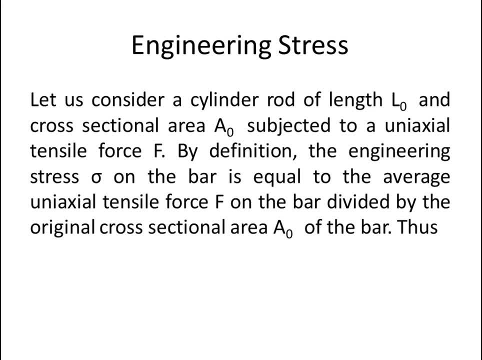 Engineering Stress. us consider a cylinder rod of length L0 and cross-sectional area A0 subjected to a uniaxial tensile force F. By definition, the engineering stress phi on the bar is equal to the FRS uniaxial tensile force F on the bar divided by the original cross-sectional area A0 of 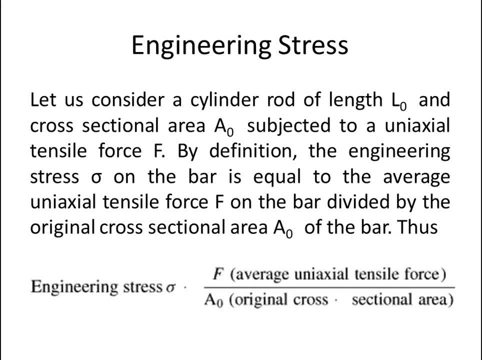 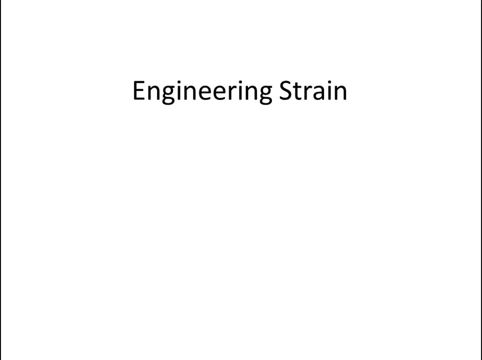 the bar. Thus engineering stress equal F by A0. F means average uniaxial tensile force and A0 means original cross-sectional area. Now let's talk about engineering strain. When a uniaxial tensile force is applied to a rod, it causes the rod to be elongated in. 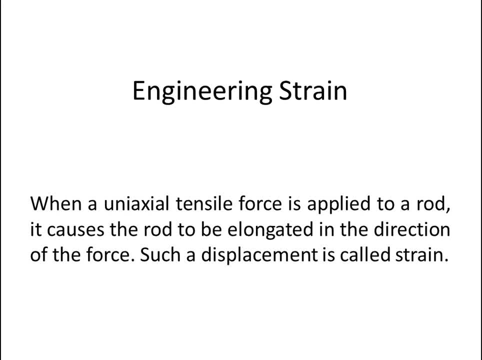 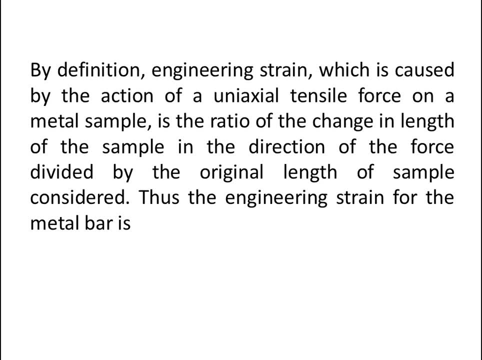 the direction of the force. Such a displacement of the uniaxial tensile force is applied to the rod. Such a displacement of the uniaxial tensile force is applied to the rod. Such a displacement is called strain By definition, engineering strain, which is caused by the. 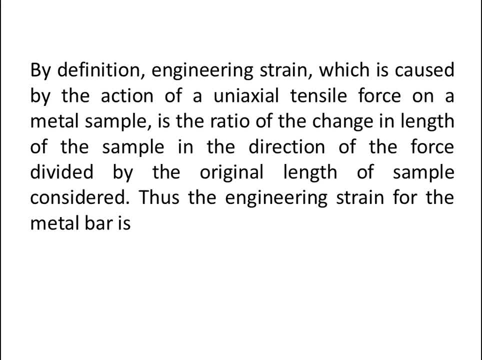 action of a uniaxial tensile force on a metal sample is the ratio of the change in length of the sample in the direction of the force, divided by the original length of sample considered. Thus, the engineering strain for the metal bar is, that is: 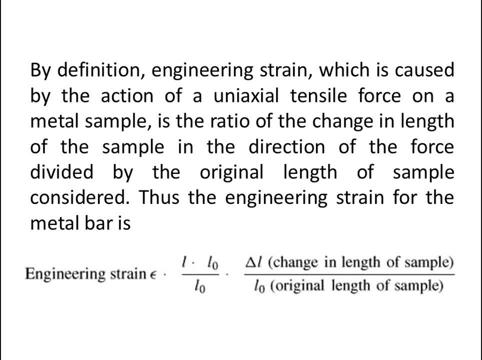 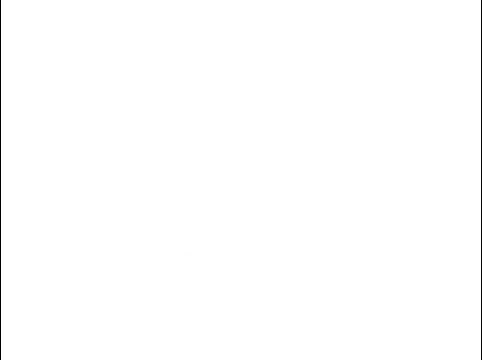 del L by L0. So engineering strain means change in length of sample by the original length of sample. And there is a sample and here the length is L0 and the cross-sectional area is A0. And when force is applied, tensile force is applied- its length increases and 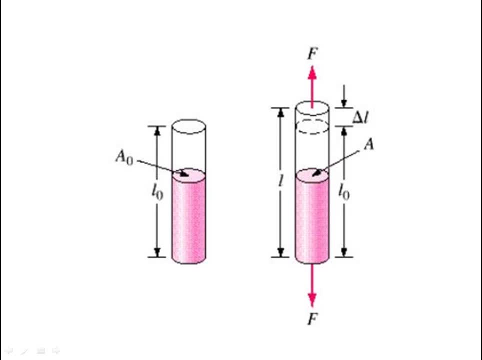 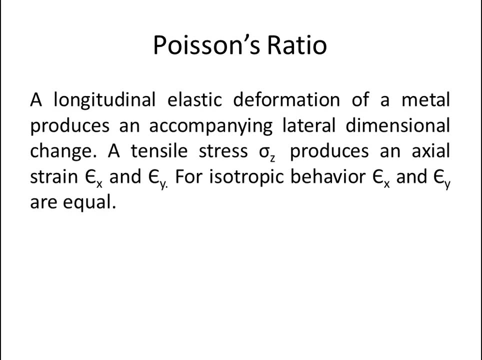 the increment is del L. Now let's talk about Poisson's ratio. A longitudinal elastic deformation of a metal produces an accompanying lateral dimensional change. A tensile stress, phi z, produces an axial strain- eta x and eta y. For isotropic behavior, eta x and eta y are equal And the Poisson's ratio is equal to. 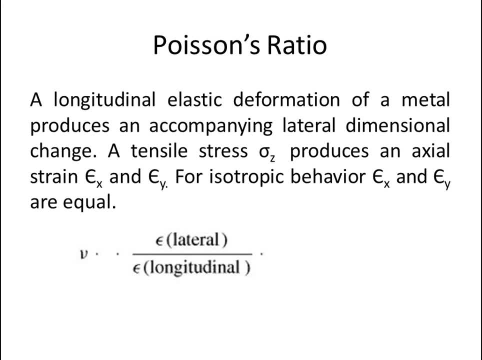 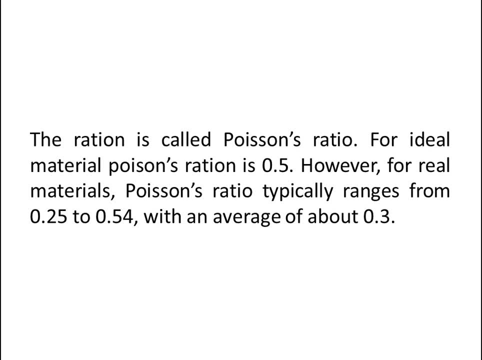 a lateral strain by a longitudinal strain. The ratio is called Poisson's ratio. For ideal material, Poisson's ratio is 0.5.. However, for real materials, Poisson's ratio typically ranges from 0.25 to 0.54, with an average of. 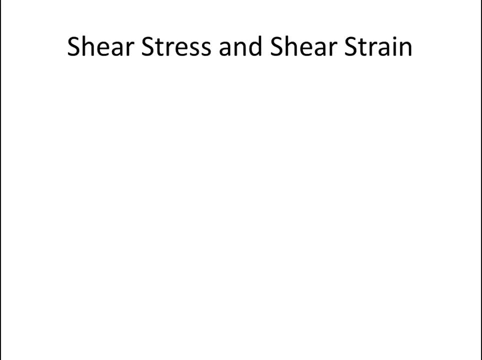 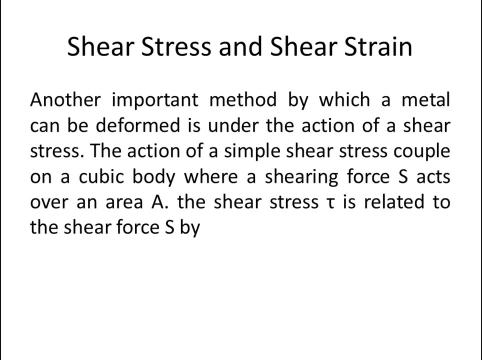 about 0.3.. Now let's talk about shear stress, Shear strain. Another important method by which a metal can be deformed is under the action of shear stress, The action of a simple shear stress couple on a cubic body where a shear force S acts. 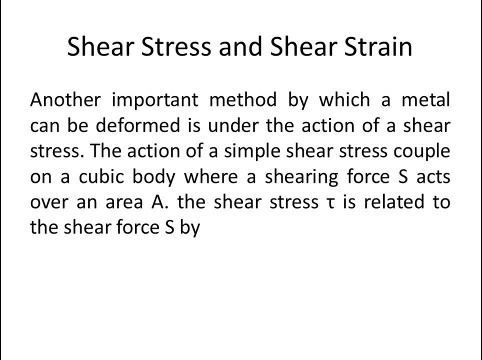 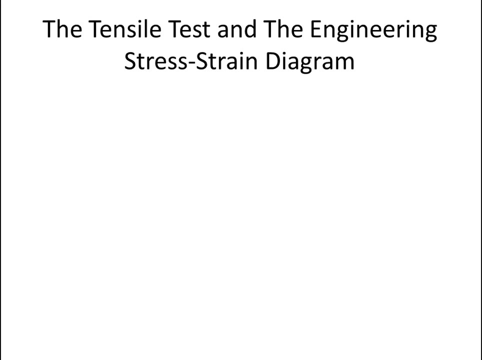 over an area A. The shear stress, tau is related to the shear force. S by the shear stress equal S by A. S means shear force and A means area over which shear force acts. Now let's talk about the tensile test and the engineering stress strain diagram. The 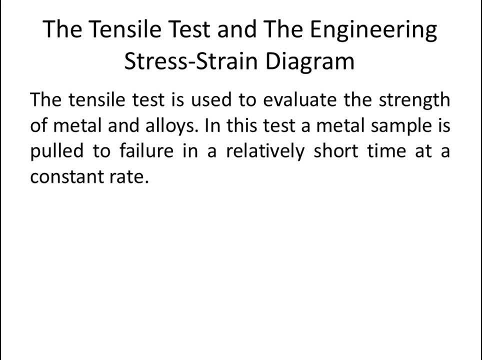 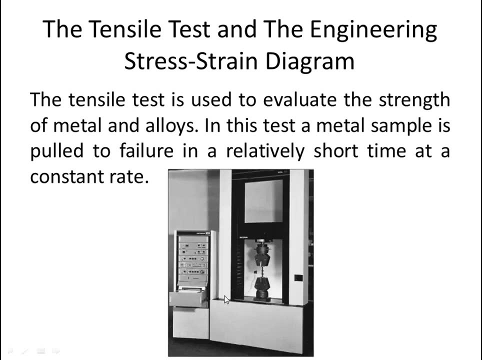 tensile test is used to evaluate the strength of metal and alloys. In this test, a metal sample is pulled to failure in a relatively short time at a constant rate. There is a machine for this test and actually end portion of the sample is cool, and by this tool the force is applied, And because of this 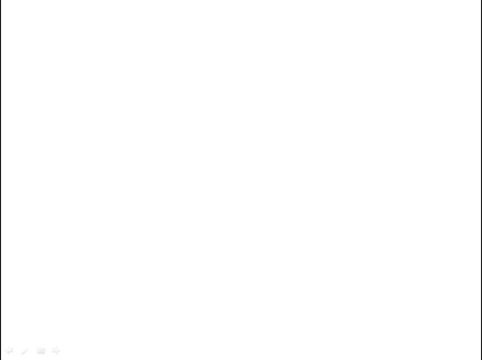 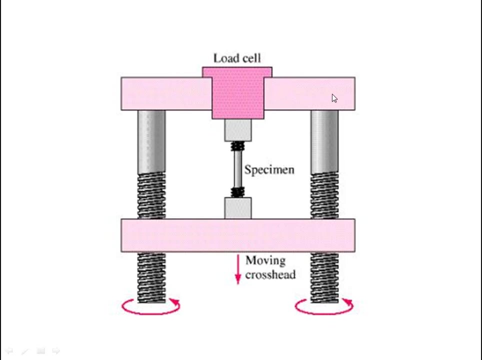 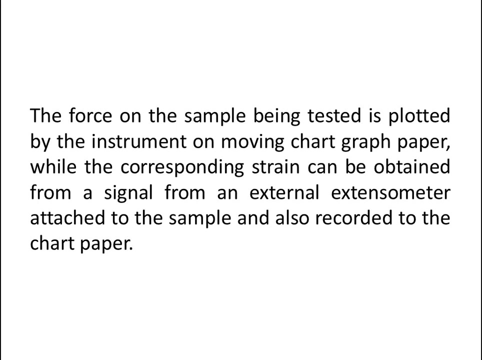 force, the metal fails. This is the diagram of the load and this is specimen, and the load cell and this is a moving crosshead and this one goes downward and because of this force this specimen fails. The force on the sample being tested is plotted by the instrument on moving chart: graph paper. 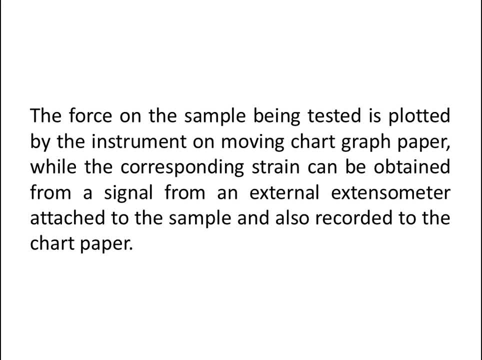 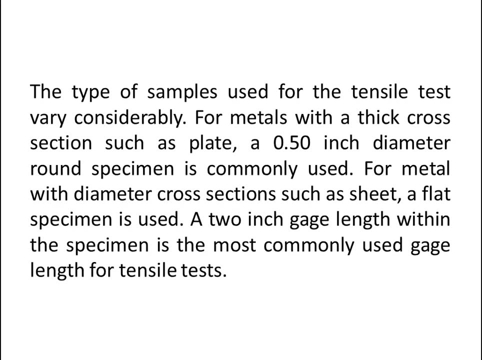 while the corresponding strain can be obtained from a signal from an external extensometer attached to the sample and also recorded to the chart paper. The type of samples used for the tensile test vary considerably. For metals with a thick cross-section, such as plate, a 0.50 inch diameter round specimen. 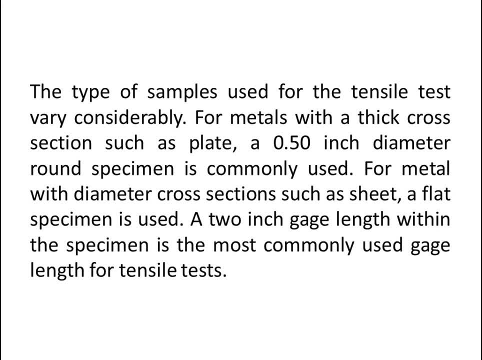 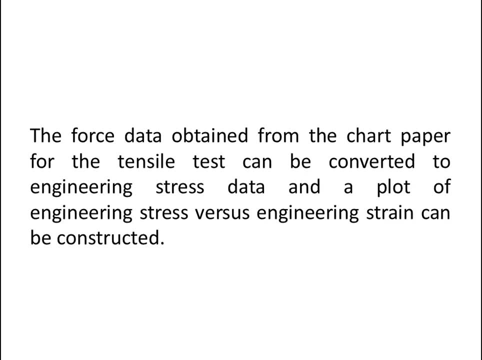 is commonly used. For metal with diameter cross-section, such as sheet, a flat specimen is used. A 2 inch gauge length within the specimen is the most commonly used gauge length for tensile test. The force data obtained from the chart paper for the tensile test can be converted to engineering. 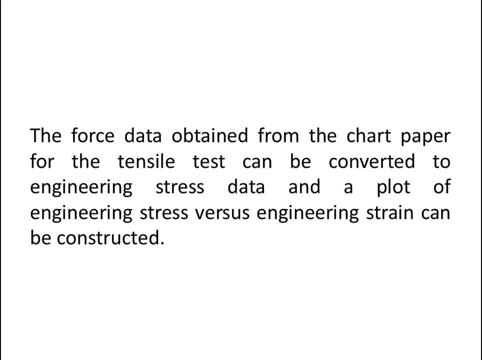 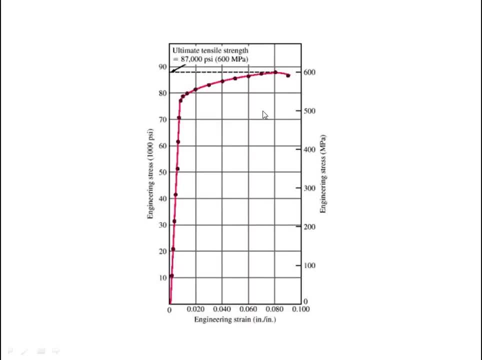 stress data and a plot of engineering stress versus engineering strain can be constructed. The growth rate in section A can be evaluated from the resultant value derived from the measurement by using order of mass and number of initial gun and area in relation to the chamber. 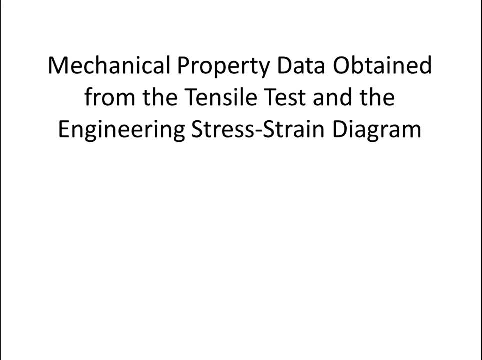 In theек portion, which can mining machine scale measurements. wereиш schöne in the previous video. this is how the sample results certificate can be obtained. Lets now move onto mechanical technique test results, which is obtained from 10-grad test and the engineering stress-train diagram. 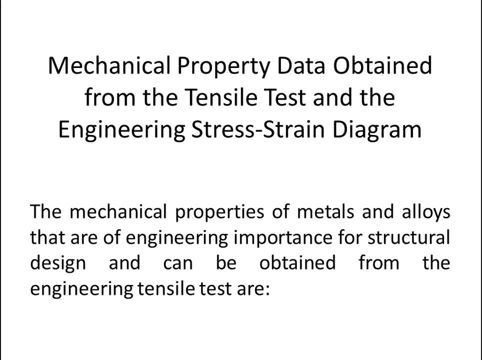 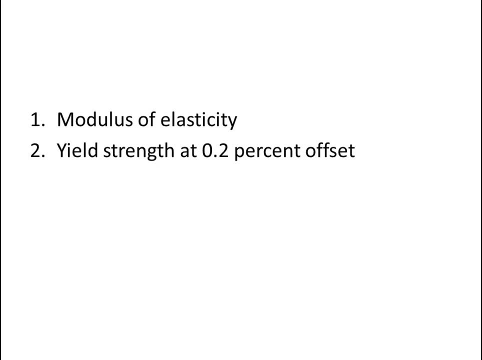 The mechanical property of the metals and insulted Первz sleizhed�� will impact the tensile test results. alloys that are of engineering importance for structural design and can be obtained from the engineering tensile tests are: first one modulus of elasticity, second one is strength at 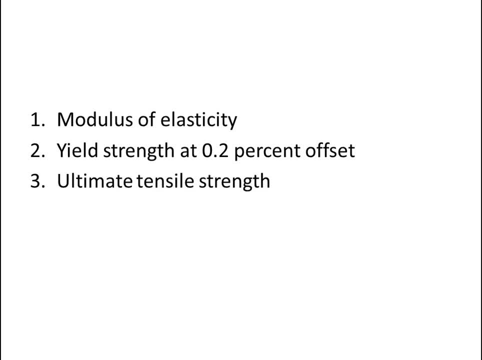 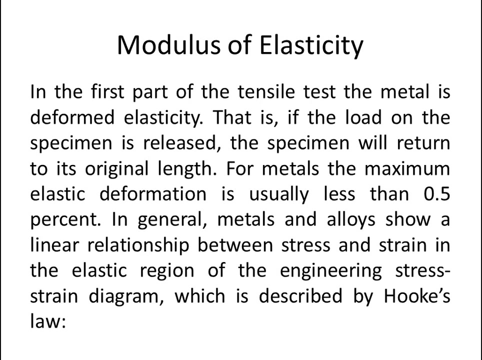 0.2 percent offset. third, one ultimate tensile strength. fourth, one percent of elongation at fracture. fifth, one percent reduction in area at fracture. now let's talk about modulus of elasticity. in this first part of the tensile test the metal is deform. elasticity, that is, if the load on the 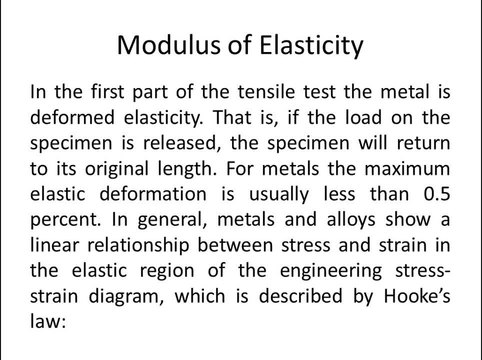 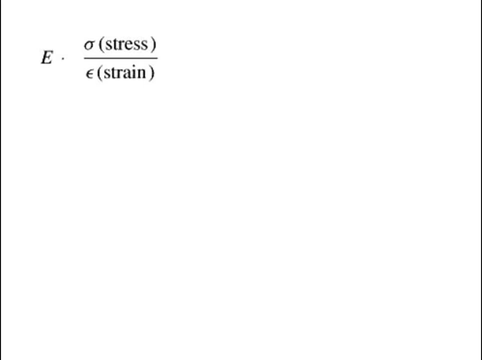 specimen is released, the specimen will return to its original length. for metals, the maximum elastic deformation is usually less than 0.5 percent. in general, metals and alloys show a linear relationship between stress and strain in elastic region of the engineering stress strain diagram, which is described by the hook's law. the hook's law is that is stress by strain. 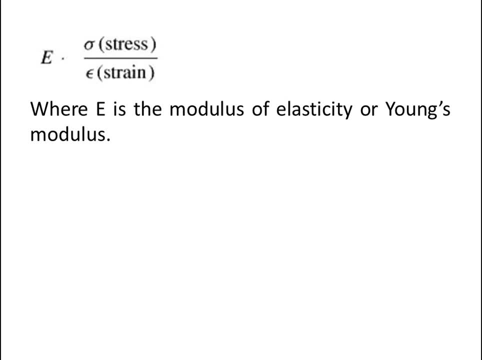 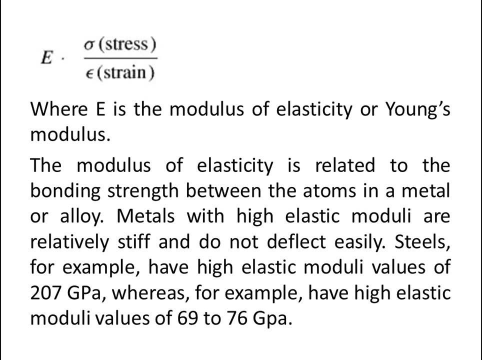 where e is the modulus of elasticity or young's modulus. the modulus of elasticity is related to the bonding strength between the atoms in a metal or alloy. metals with high elastic modulus are relatively stiff and do not deflect easily. steels, for example, have high elastic modulus values of 207 giga pascal. higher, for example, have 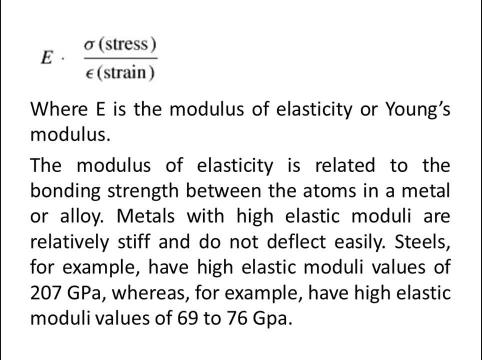 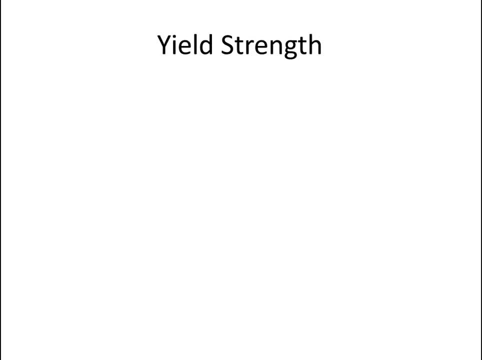 high elastic modulus values of 69 to 70, value of shielding of deepest range, and abbiamo mill� not highly elastic medals in more than one thousand of thefields" 76 Giga Pascal. Now let's talk about L strength. The L strength is a very 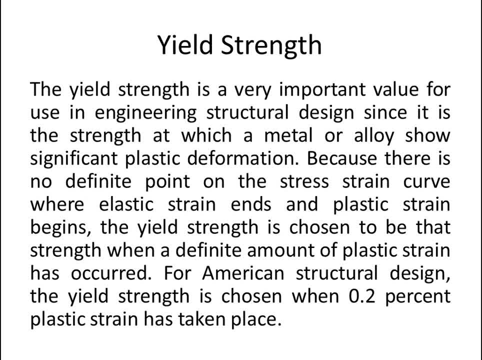 important value for use in engineering structural design, since it is the strength at which a metal or alloy shows significant plastic deformation. Because there is no definite point on the stress strain curve where elastic strain ends and a plastic strain begins, The L strength is chosen to be that strength when a 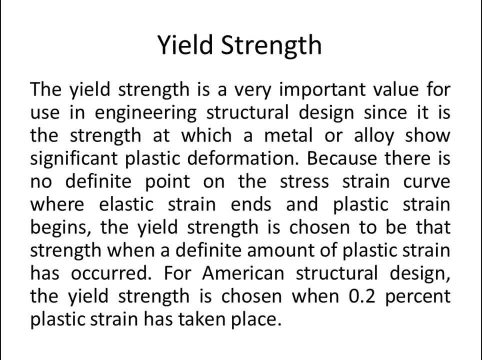 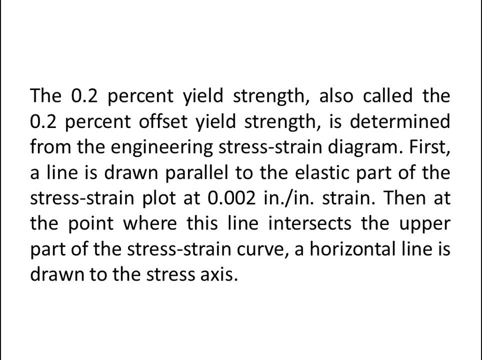 definite amount of plastic strain has occurred. For Americal structural design, the L strength is chosen when the 0.2% plastic strain has taken place. The 0.2% L strength, also called the 0.2% offset L strength, is determined from the engineering stress. 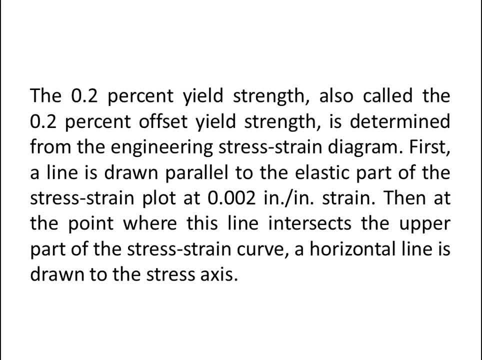 strain diagram. First, a line is drawn parallel to the elastic part of the stress strain plot, at 0.002 inch by inch strain. Then, at the point where this line intersects the upper part of the stress strain curve, a horizontal line is drawn to the stress axis. 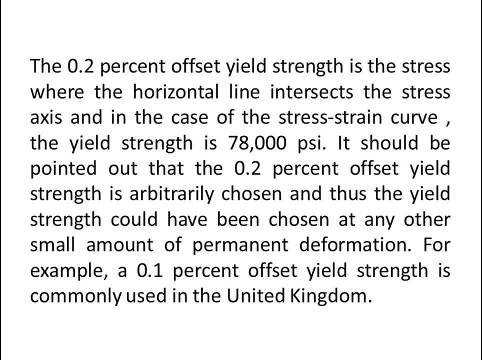 The 0.2% offset L strength is the stress where the horizontal line intersects the stress axis and in the case of the stress strain curve, the L strength is 78000 psi. It should be pointed out that the 0.2% offset L strength is 0.2% offset L strength. 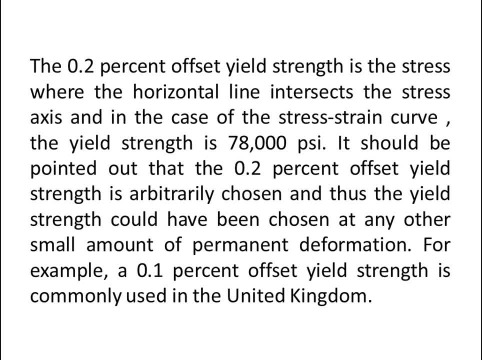 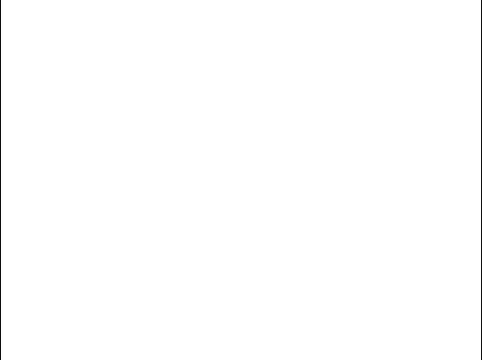 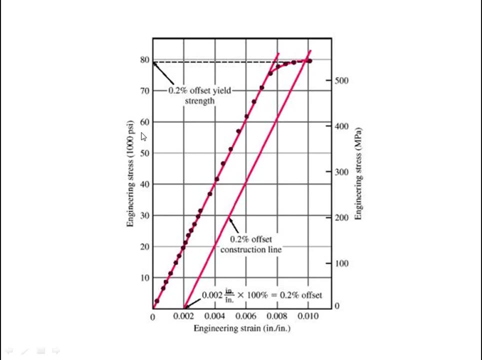 The 0.2% offset L strength is arbitrarily chosen and thus the L strength could have been chosen at any other small amount of permanent deformation. For example, a 0.1% offset L strength is commonly used in the United Kingdom And this is the figure So vertical there is engineering stress. 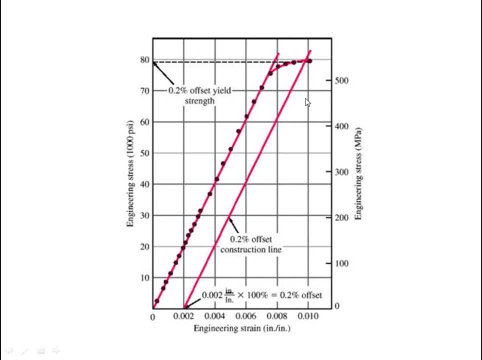 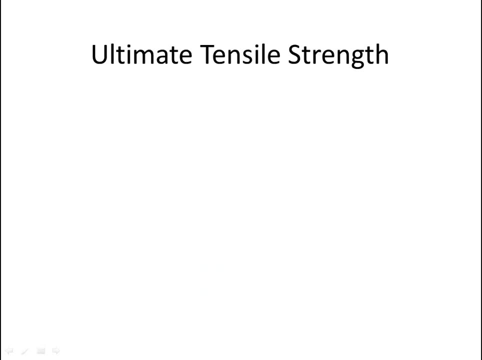 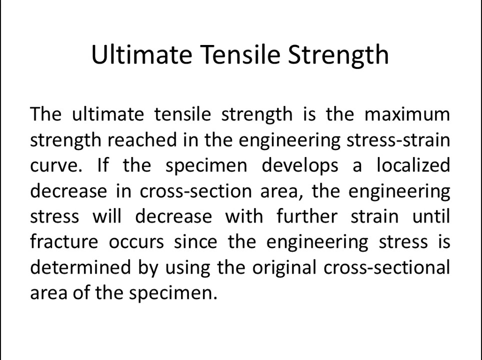 and horizontal, there is engineering strain And this line is the actually 0.2% offset construction line and this is our linear relation between stress and strain. Now let's talk about ultimate tensile strength. The ultimate tensile strength is the maximum strength raised in the engineering stress. 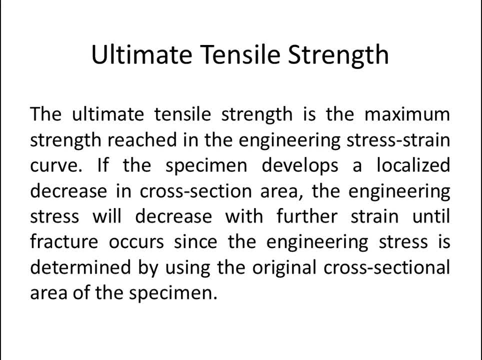 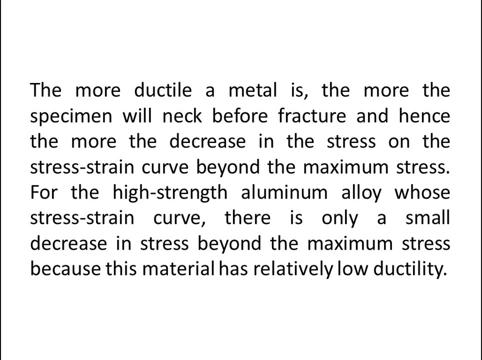 strain curve. If the specimen develops a localized decrease in cross-section area, the engineering stress will decrease with further strain until fracture occurs, since the engineering stress is determined by using the original cross-sectional area of the specimen. The more ductile a metal is, the more the specimen will neck before fracture and hence the more the 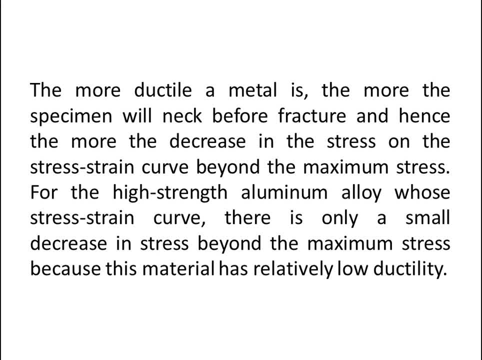 decrease in the stress on the stress strain curve beyond the maximum stress. For the high strength aluminum alloy, whose stress strain curve, there is only a small decrease in stress beyond the maximum stress because this material has relatively low ductility, An important point to understand with. 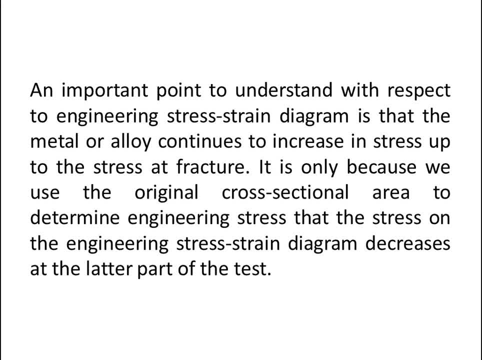 respect to engineering stress-strain diagram is that the metal or alloy continues to increase in stress affords stress at fracture. It is only because, while the stress is determined by the, we use the original cross sectional area to determine engineering stress that the stress on the engineering stress strain diagram decreases at the later part of the test.